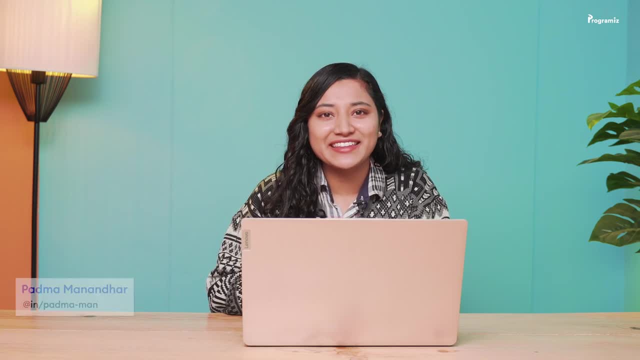 What's up guys? Welcome back to this series on C programming. In this video we'll learn about pointers in C. More specifically, we'll learn to work directly with computer memory address with the help of pointers. So let's get started. 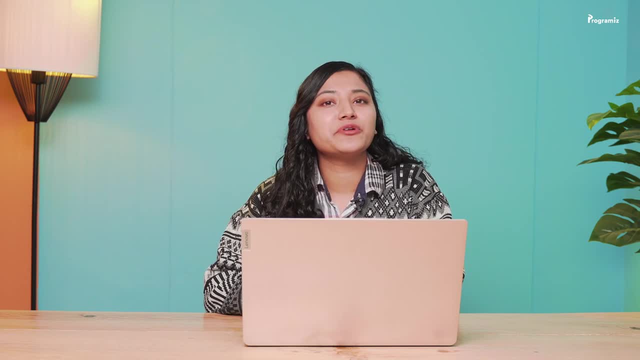 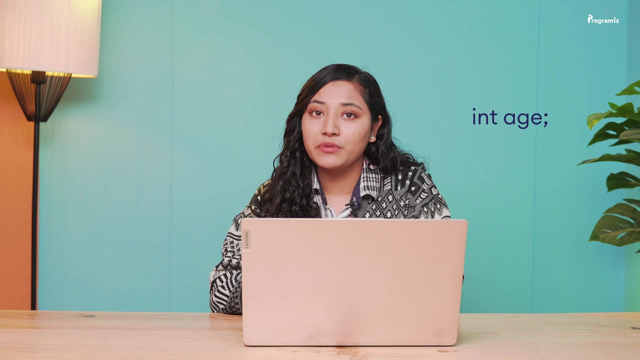 Pointer is one of the main features that make C programming so powerful. It allows us to work directly with the computer memory. Before we learn about pointers, let's first learn about addresses In C programming, whenever we declare a variable, a space will be allocated in the memory for the variable and C allows us to access the address of the variable. 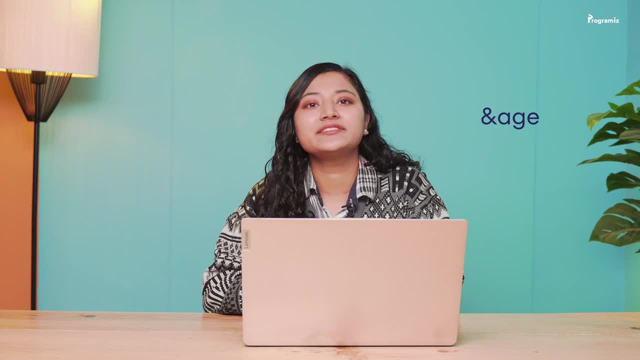 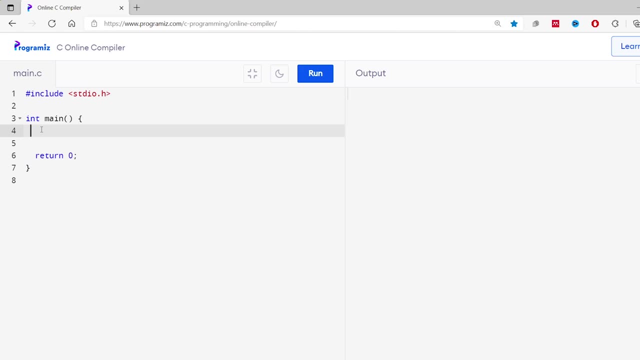 We use the ampersand symbol with the variable name to access the memory address. Let's see an example. You might be familiar with the basic structure of C program. Now I'll create an. int is, a variable is, So int is, and I'll assign value 25 to this. 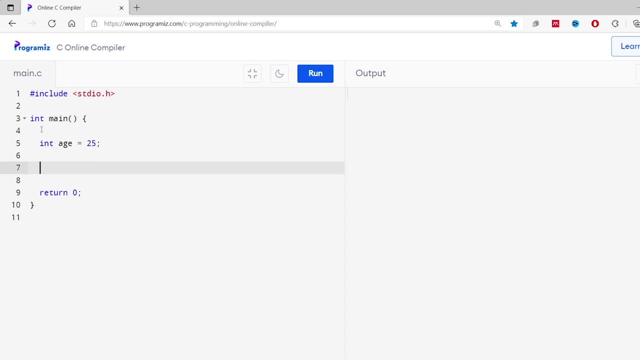 Now let's use ampersand symbol to access the address where the is variable is stored. So printf: %p. ampersand is Here. I have used %p format specifier to print the address. Now let me run this code. 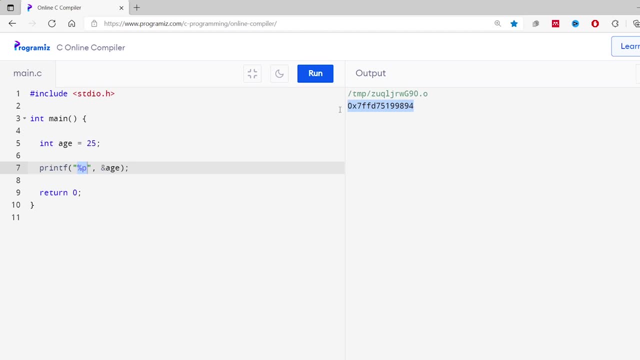 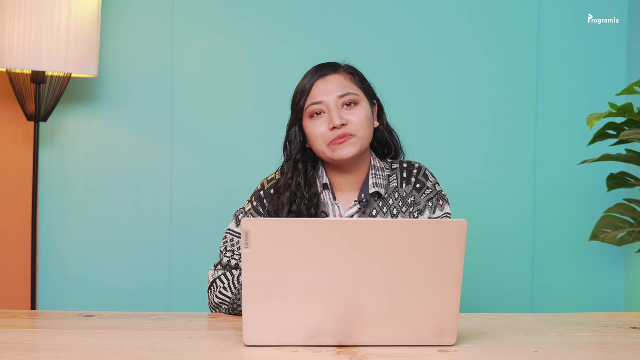 Here you can see we get this output, which is the memory address where 25 is located. When you copy and run the exact same code, you may get different output, because the output is based on the location where the variable is stored and it varies device to device. 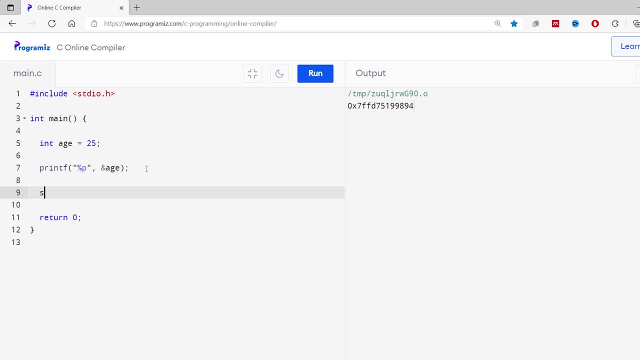 If you remember, we have used ampersand symbol with scanf like this, like ampersand is So usually we use this ampersand is with scanf while taking input from the user. This is because with scanf, we are instructing the compiler to store the input value at the memory address specified by this ampersand is. 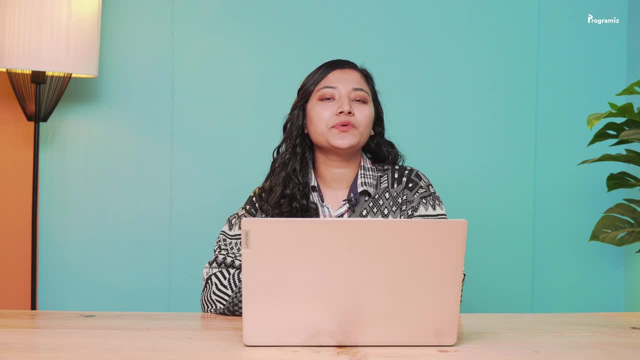 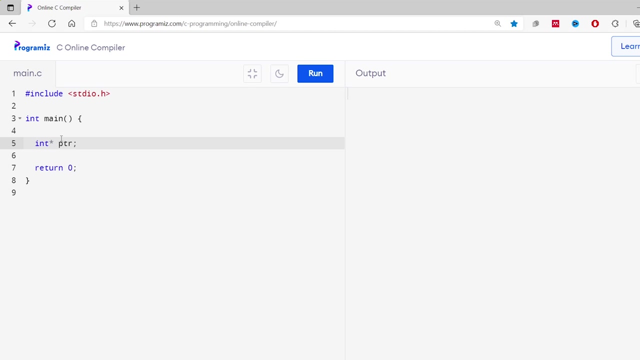 Scanf from compiler. Now that you know about memory addresses, let's get back to pointers. Just like a regular variable, a pointer is also a variable variable stores the memory addresses of the variable, not the actual value. Let's now see how we can create pointers. So I'll create pointer int, asterisk, ptr. Here ptr is a pointer variable. 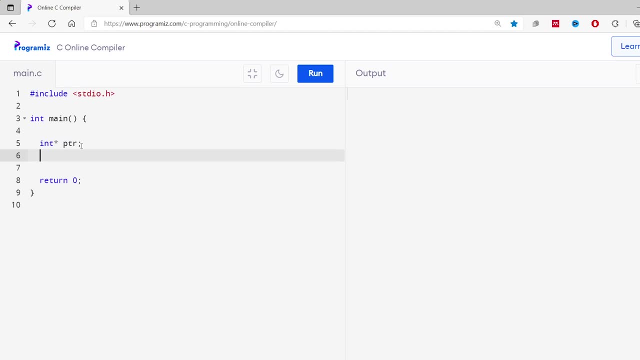 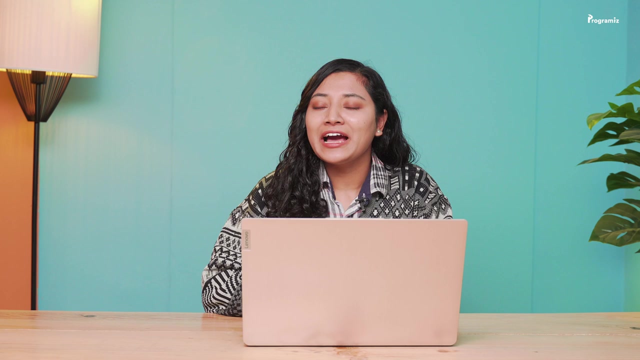 Let me create a regular variable and compare these two. So I'll create int var. When comparing these two, you can see the only difference between these two is this asterisk symbol. Now let's see how we can assign value to a pointer variable. Here is our code from our earlier program Now. 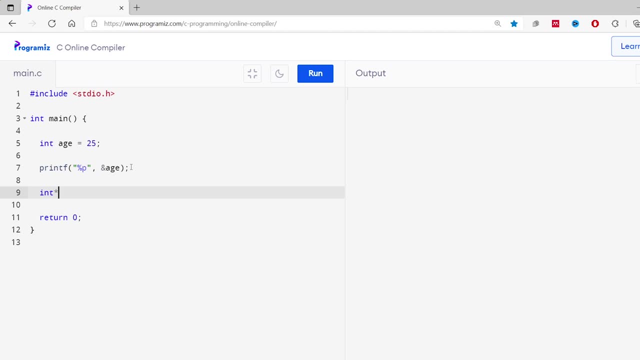 let me create a pointer variable: int, asterisk, ptr. As we know, a pointer variable stores a memory address of a variable and we also know that ampersand is gives the memory address. So when we assign a pointer variable to a variable, it stores a memory address of a variable. So we 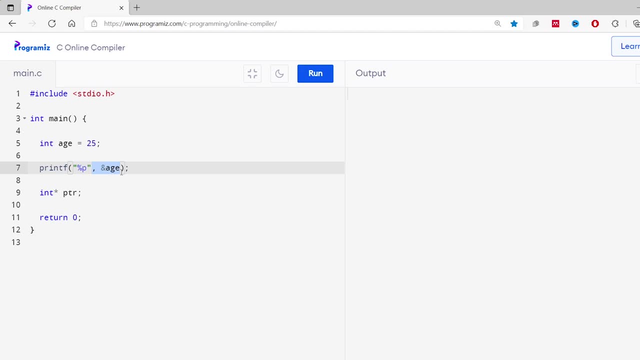 assign ampersand is to the pointer variable. The pointer variable should store the memory address of the is variable. So let's do that Now. I'll assign this pointer to the address of is variable and I'll print this using printf statement comma ptr. 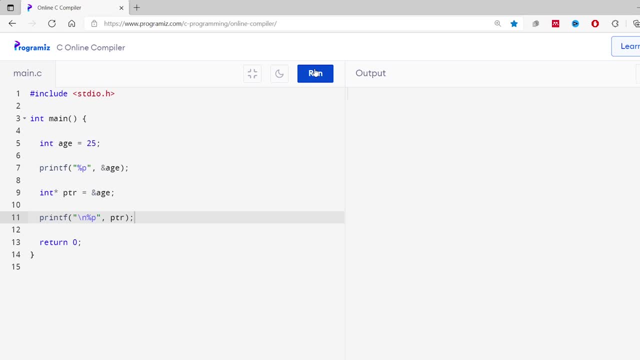 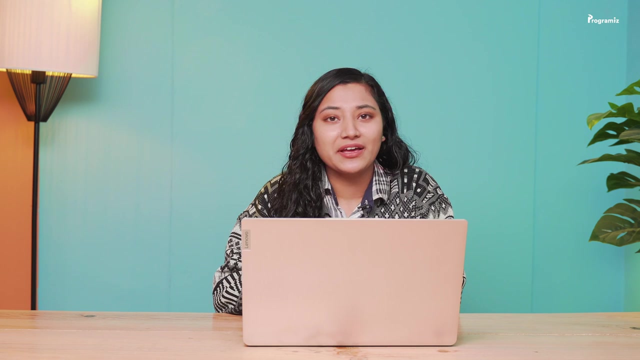 Now let me run this code Here. you can see we get the same result for both ampersand is and ptr. By the way, if you're watching this, there is a good chance. you want to improve your skills in C programming. Lucky for you, we have a mobile app that provides a well-structured C programming course. 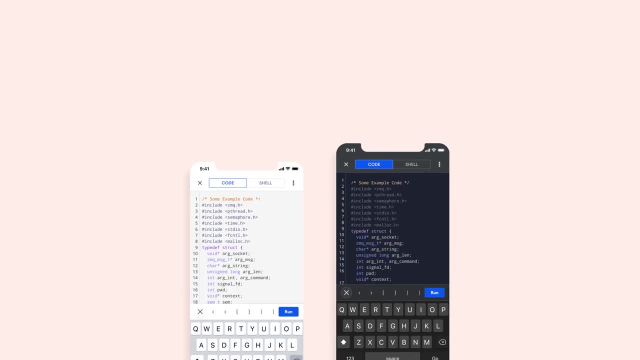 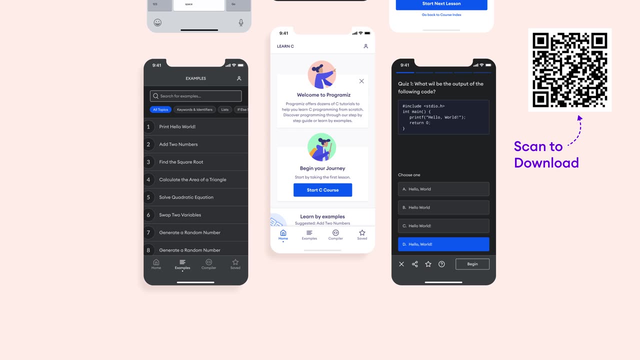 with certification at the end, and you can use the app alongside the video to practice on the Vuelden compiler. Our course is free, so you don't have to worry about it. So let's get started. So download now by scanning this QR code or click the link in the video description. 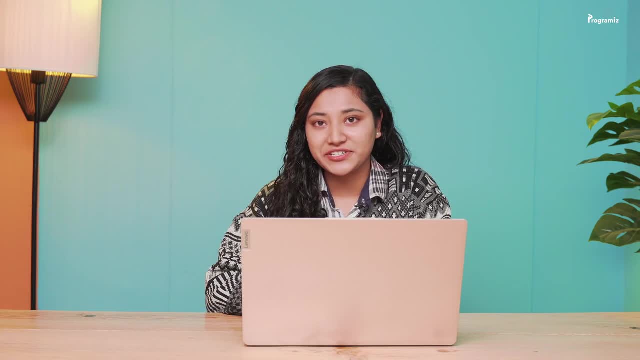 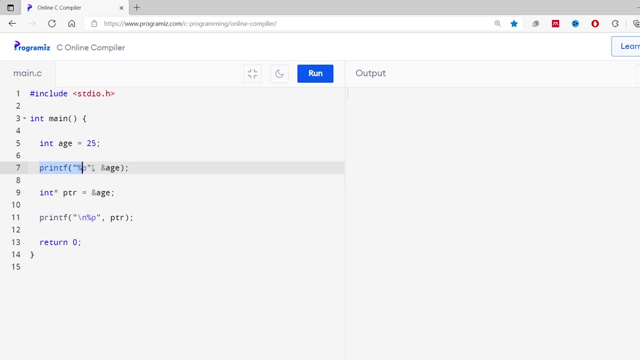 We can also access the value of a variable using the pointer. Let's see an example In our code from our earlier example. I'll remove this print statement and I'll modify this print statement here. address colon: express n. Now let's print the value using ptr pointer. I'll use printf statement printf. 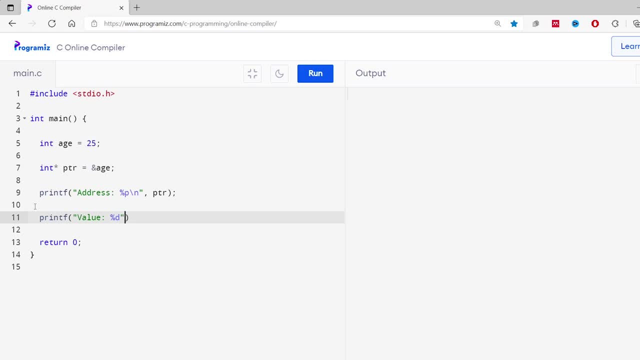 value colon, %d comma, asterisk ptr. Here asterisk ptr gives the value stored in the ptr address and since the value is in integer, I have used %d format specifier. Now let me run this code. As you can see, we have successfully accessed the value using the pointer variable. 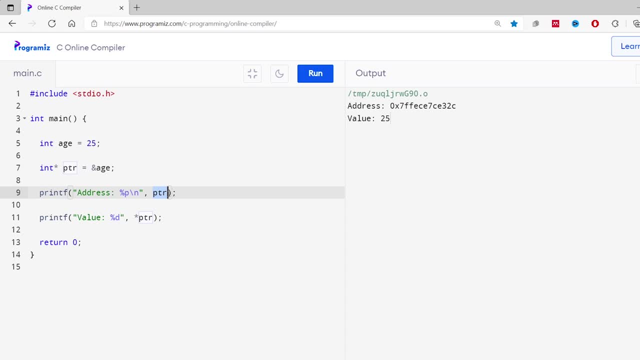 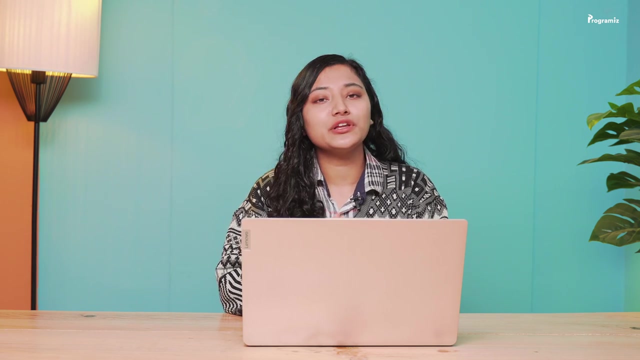 Remember, ptr is a pointer that stores the memory address and asterisk ptr gives the value stored in the memory address pointed by this ptr. In our last example we saw that we can access value of a variable using pointer variable. Similarly, we can also change the value of a variable using pointer variable. Let's see an. 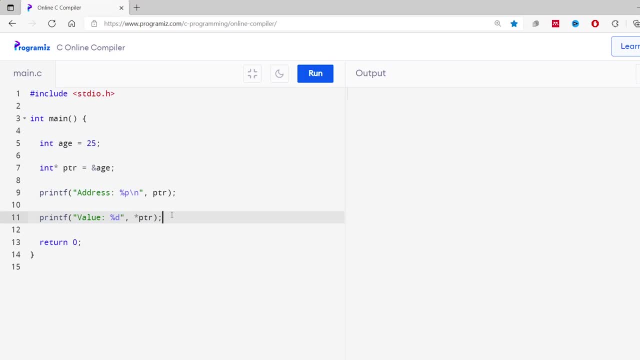 example. Here we have our code from our earlier program. Here in this program I'll remove these two print statements. Now let's use pointer variable to change the value from is 25 to 31.. So I'll use pointer and assign value 31.. Since we know asterisk ptr gives the value pointed by the 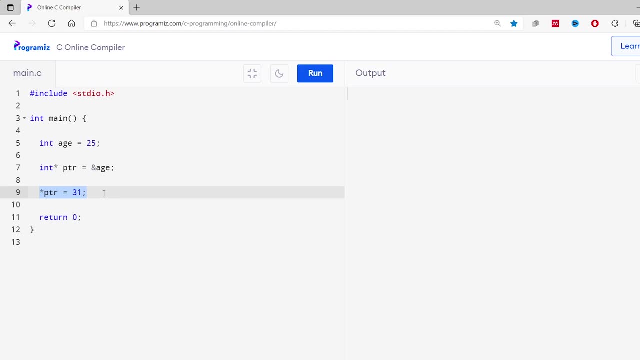 ptr address. So this code assigns a new value to the memory address pointed by the PTR variable. now let's print the value of the is variable. I'll use printf statement- percent D comma is, and I'll run this here you can see the value of is variable is changed. 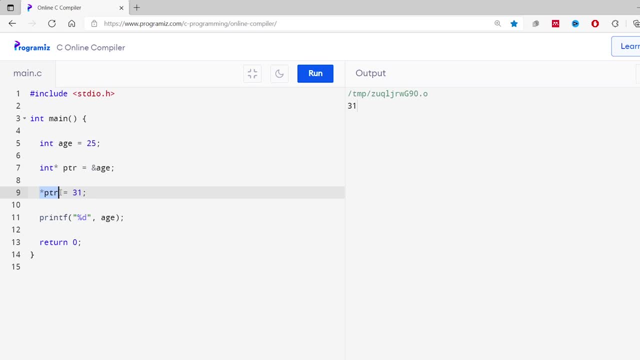 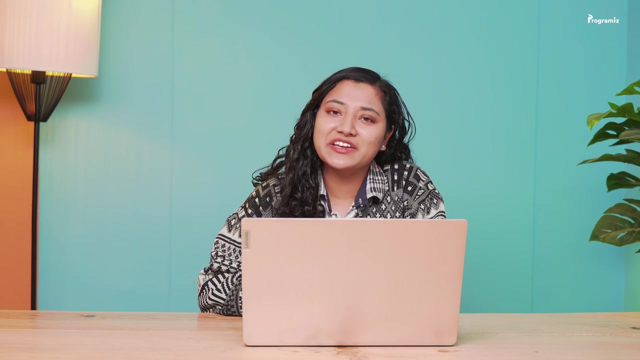 to 31. this is because the PTR pointer points to the address of is variable and we have changed the value pointed by PTR pointer from 25 to 31. so, ultimately, we have changed the value of the is variable. ok, guys, we need your support to keep these types of content free for all users. YouTube really likes engagement on. 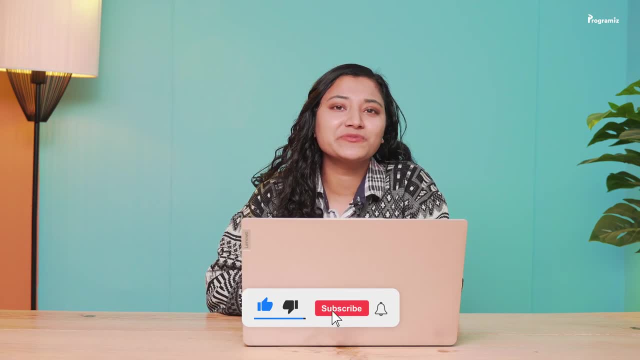 the video. so leave a comment below, press that like button and hit subscribe. if you haven't already done so, please subscribe to our channel and hit the bell icon so you don't miss our next video already. let's get the engagement score high up so that more people can discover. 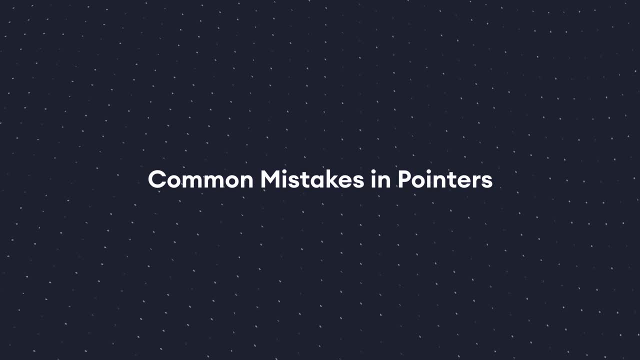 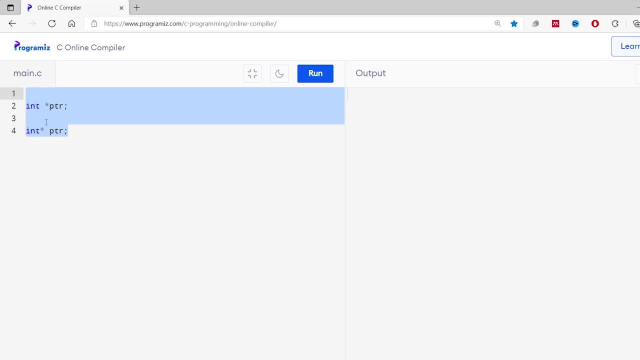 and enjoy these courses. while working with pointers, you might encounter these two syntax of creating pointers. while both are the valid ways to create pointers, you should try to avoid the first one, because this syntax sometimes creates a lot of confusion. let's try to understand this with the help of an example here we have created. 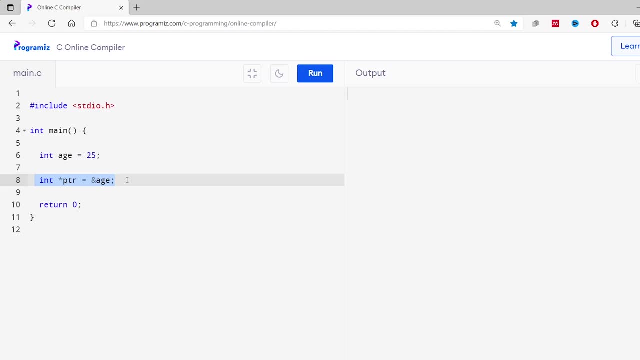 a pointer that stores the memory address of is variable and we have created a pointer that stores the memory address of the is variable. in this syntax, this asterik symbol is attached to PTR- so many things- that this asterik PTR is the pointer and try to print the address using asterik PTR, which is wrong. this is because asterik 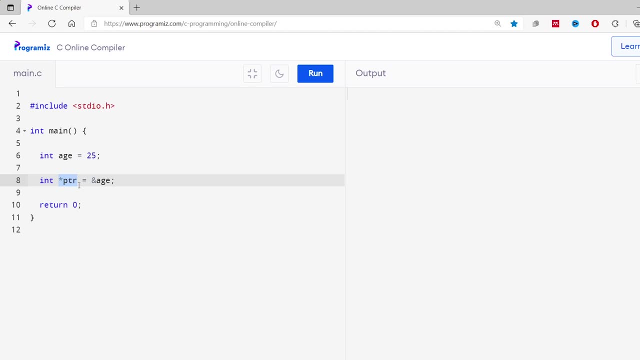 PTR gives the value pointed by the pointer, not the memory address. let me show you. I'll use printf statement: your%d asterik ptr. let's go back to the ptr and I'll run this. As you can see, we get the value of the as variable, not the memory address. 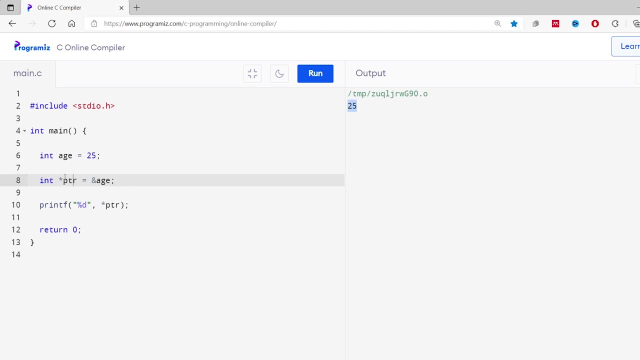 So to avoid this confusion, I highly recommend you to create pointer like this: Now you can visualize ptr separately as pointer and asterisk as the part of syntax to create a pointer. Now let's revise pointers. Here we have a regular variable number and pointer. 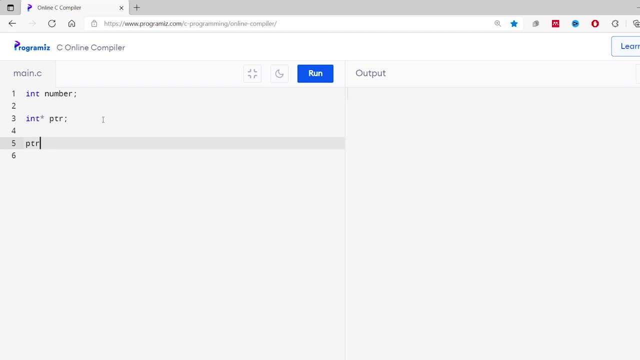 ptr, then ptr is equals to number is wrong. This is because ptr is pointer, which can only store memory address, but number is not a memory address, So this is invalid. Asterisk ptr equals to ampersand number is also wrong. This is because asterisk ptr gives the value. 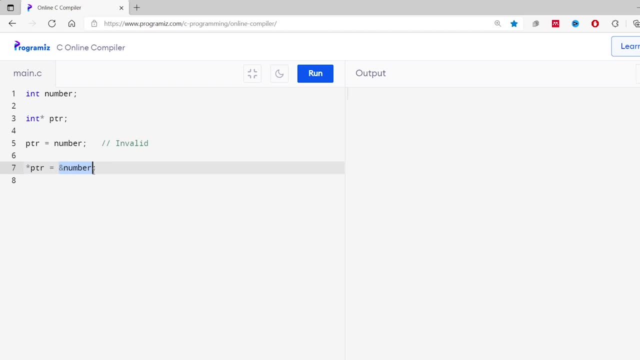 stored in the ptr location. however, ampersand number gives the memory address, So this is also invalid. Ptr equals to ampersand number is a valid code because ptr is a value stored in the ptr location. So this is also invalid. Ptr equals to ampersand number is a valid code because: